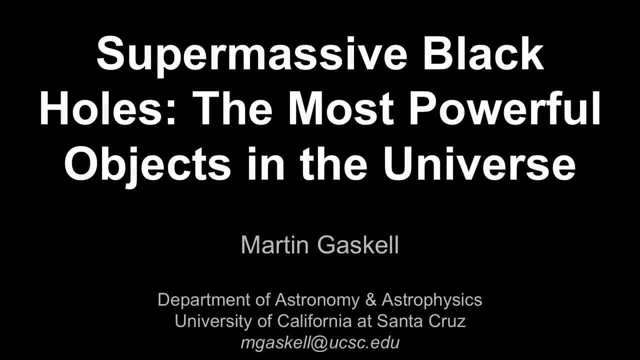 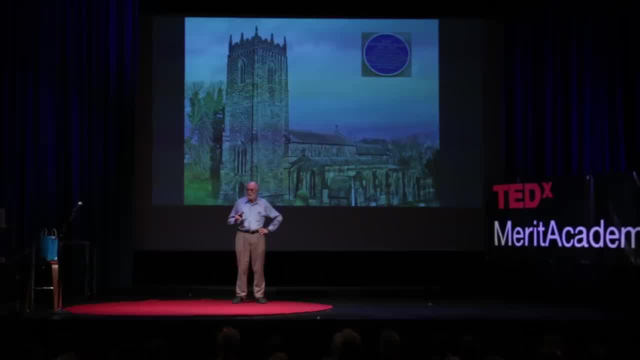 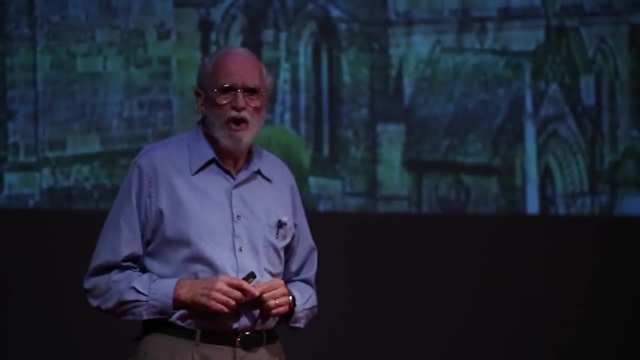 In the year 1783, a famous British scientist called the Reverend John Mitchell, the rector of this church in Thornhill, Yorkshire, presented a paper to the Royal Society in London. In his paper he argued that there could be in space, possibly, objects whose gravity was so strong. 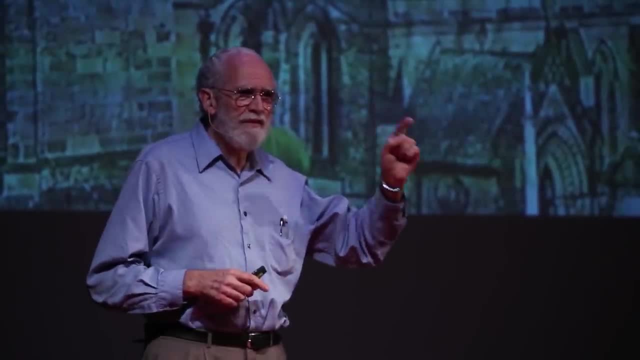 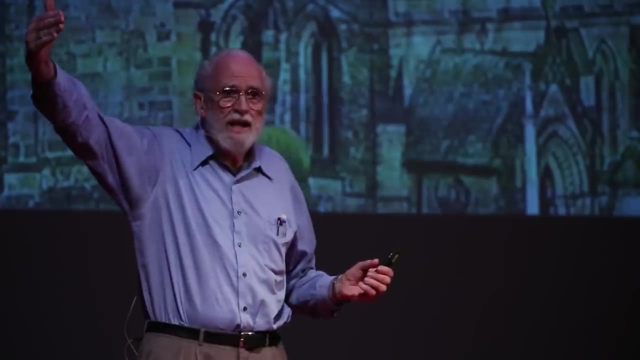 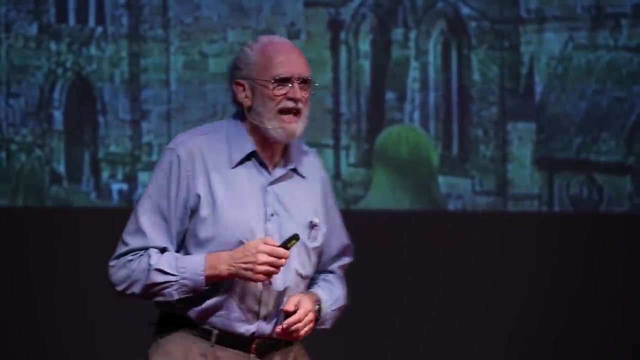 that you could not escape from them, even if you went as fast as the speed of light. And, of course, if light could not escape, then someone on the outside was not going to be able to see the object. The Reverend Mitchell had become the first person to possibly. 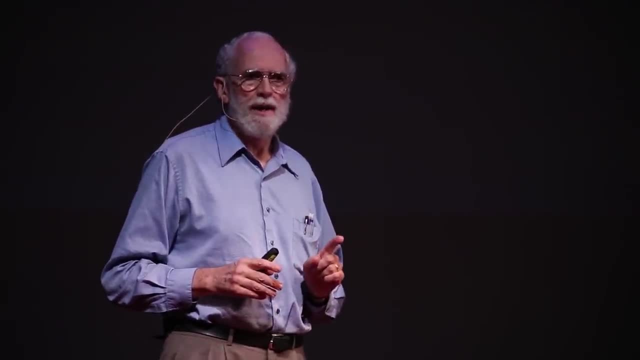 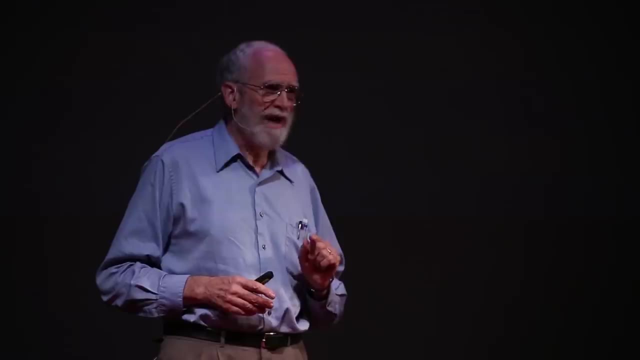 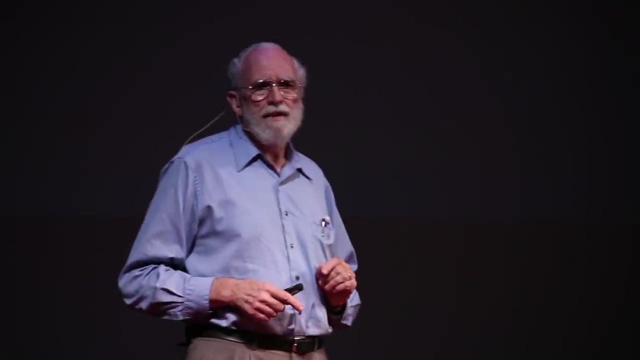 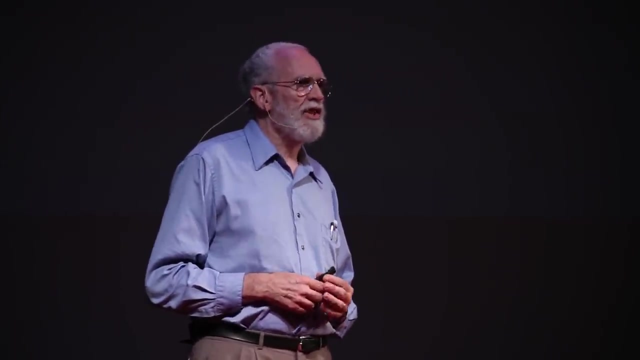 postulate the existence of what we now call black holes. Now, John Mitchell had used Isaac Newton's theory of gravity, a theory which we now know is not accurate when gravity is very strong. But in 1958, an American physicist called David Finkelstein used Albert Einstein's 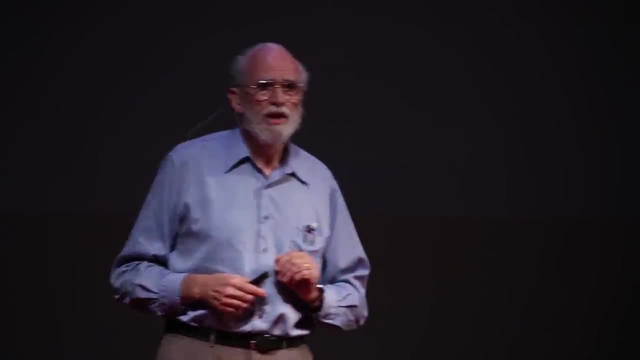 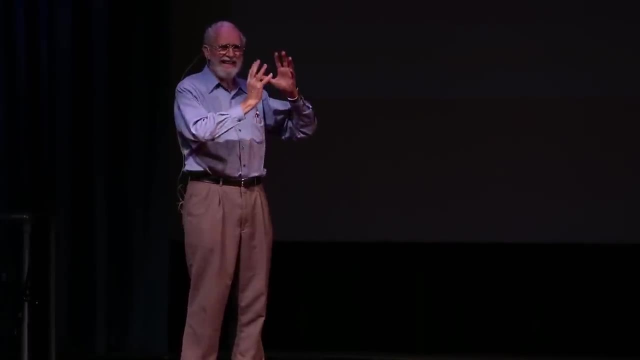 general theory of relativity, a much more accurate theory of gravity, to prove that black holes were not so strong. The black holes could indeed exist, Even though light can't escape from the black hole. the black hole has still got gravity, so it can be detected by its gravitational influence. 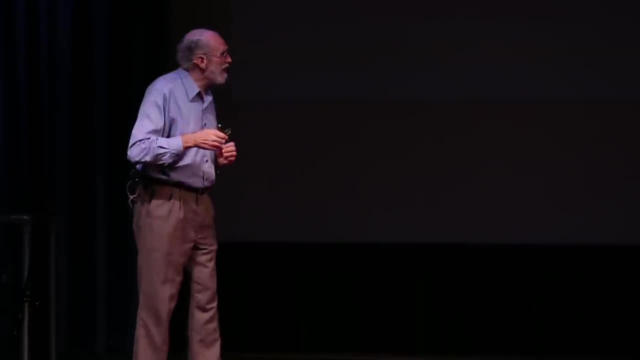 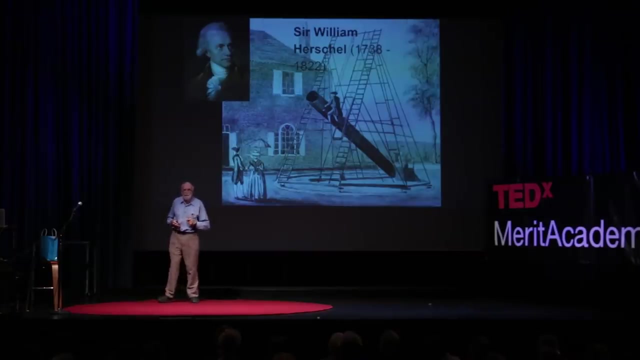 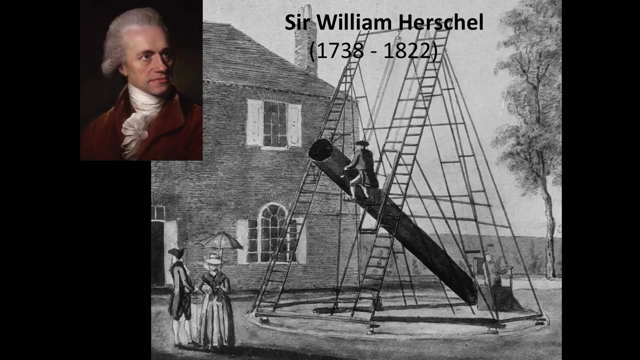 on things around it. Now, coincidentally, back in the 1780s, while John Mitchell was speculating about the existence of black holes, a friend of his, a composer called William Herschel, was using very large homemade vacuoles. 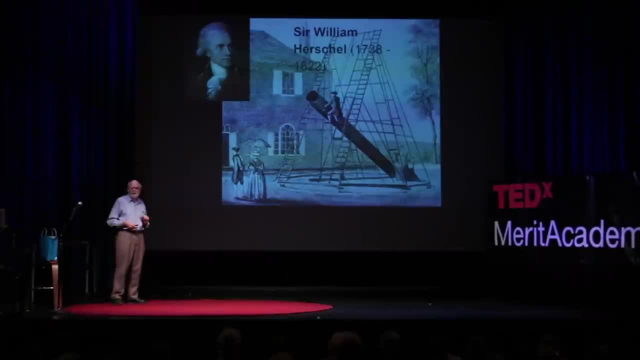 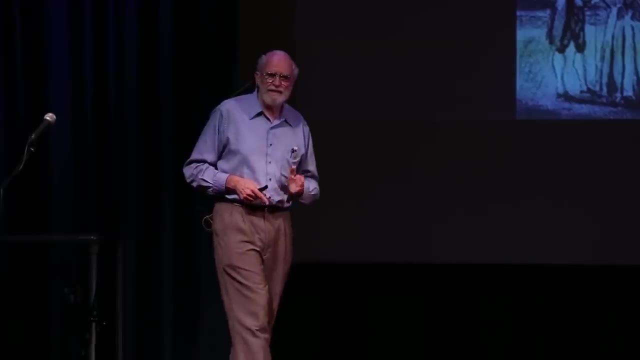 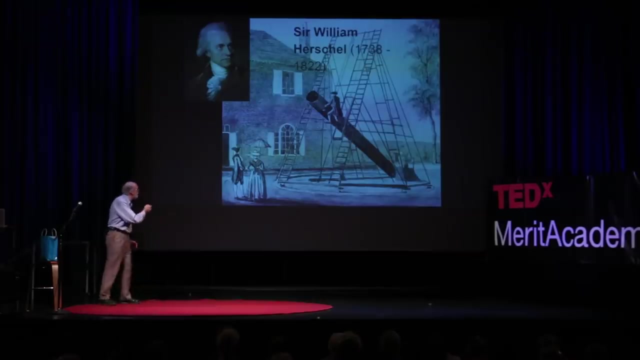 They were telescopes to sweep the sky and discover objects that we now recognize as being distant galaxies, And in some of these, in the very center we call the nucleus, he detected bright points of light. Here's a picture of one of those ones. We call it NGC. 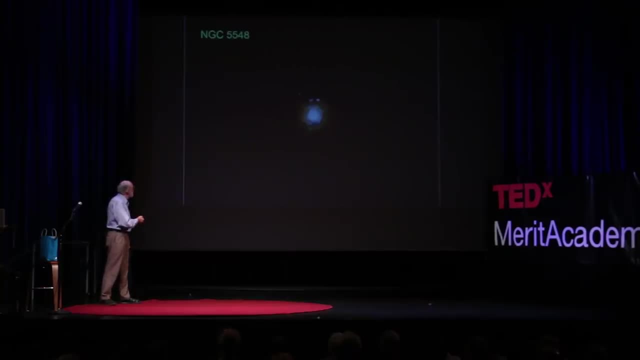 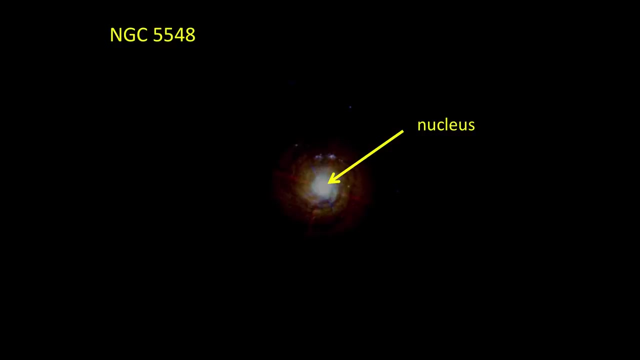 5548.. This is a Hubble Space Telescope picture of it and you can tell it's very bright in the middle, in what we call the nucleus, the center of the galaxy, And it's very bright there. William Herschel had no way of knowing this, but he was seeing light. 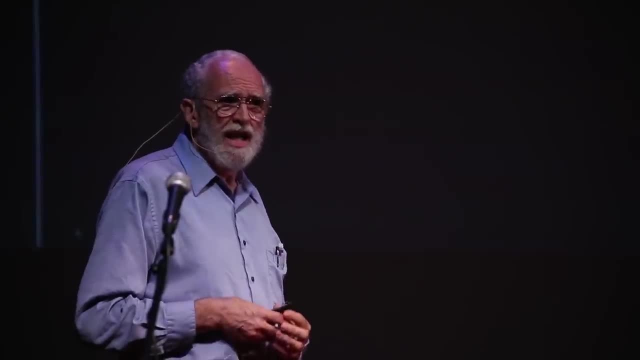 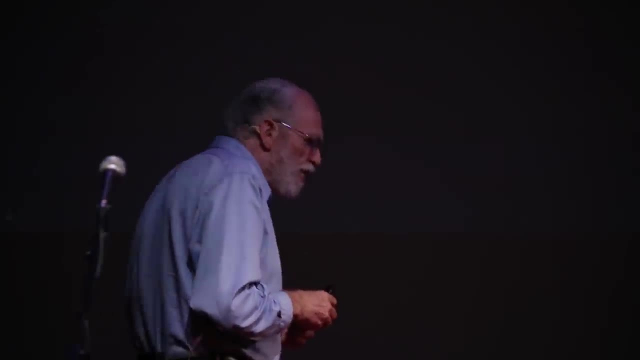 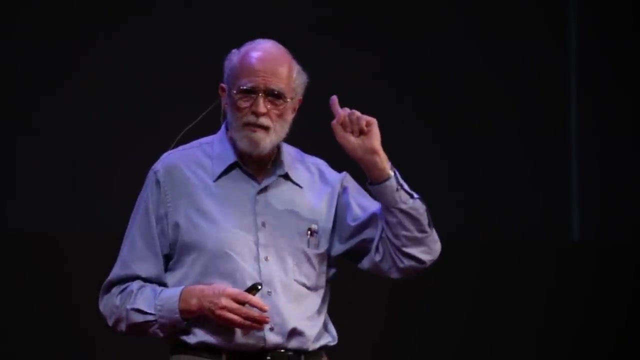 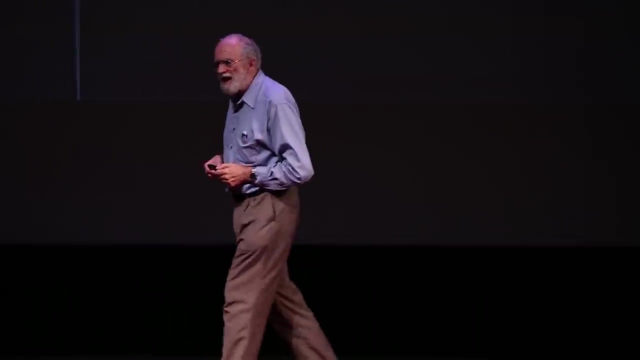 being emitted not by stars in the galaxy there, but by gas spiraling into a supermassive black hole. It was not until the beginning of the 20th century that astronomers got more indications that something bizarre was happening in the nuclei of galaxies like NGC 5548.. Astronomers at Lick Observatory. 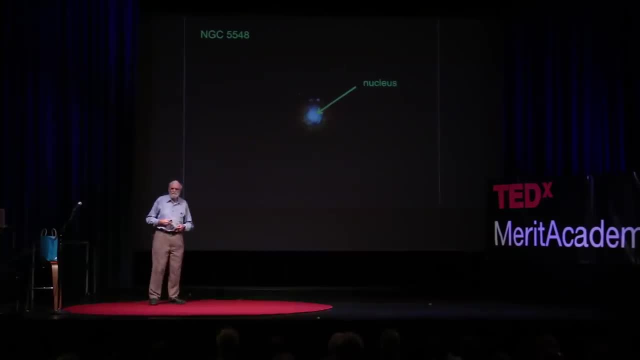 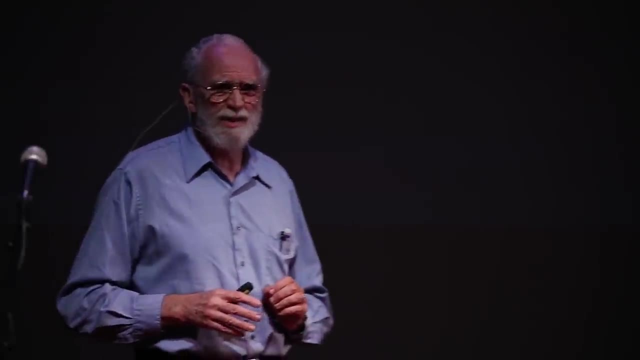 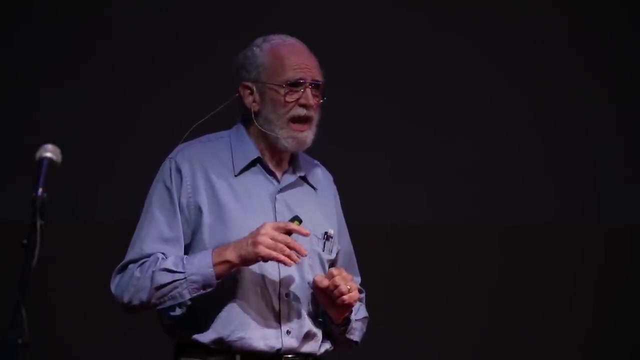 analyzed the light coming out of the nucleus of this galaxy and discovered that there was lots of hot glowing gas there and, remarkably, this gas was moving very quickly. It was moving much faster than the stars were in the galaxy. In fact, it was even going up to a few percent of the speed of light Over the next couple. 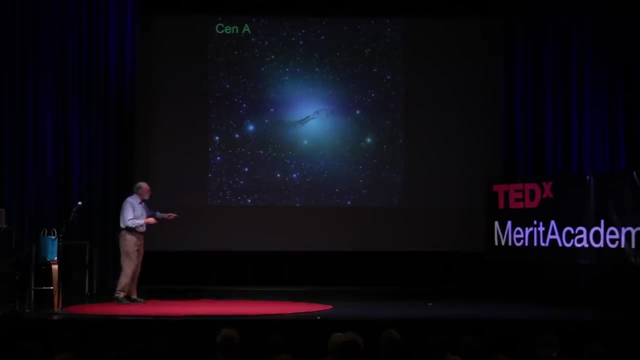 of decades, astronomers began to detect radio emission from galaxies such as this one here called Sen A, and that radio emission was very powerful. In the mid 1950s, the husband-wife team of Jeffrey and Margaret Burbage calculated that the energy being put out by an active galactic nucleus in something like Sen A 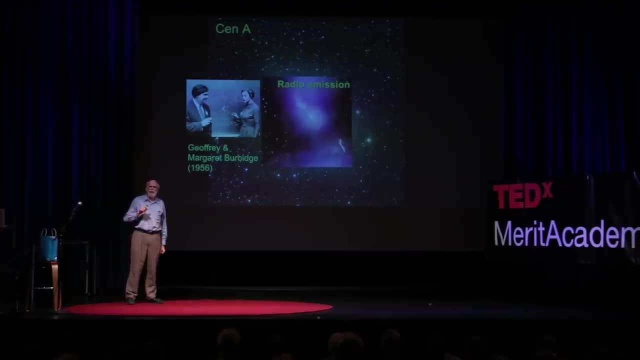 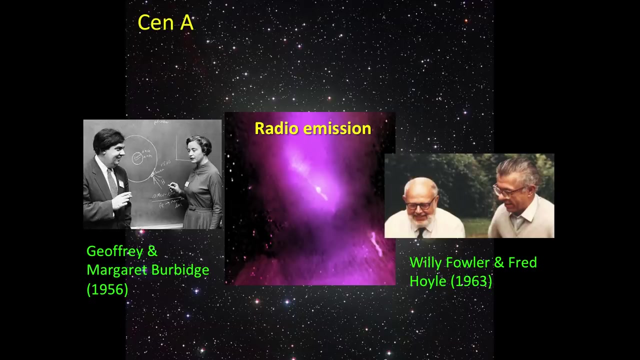 was the equivalent of 100 million supernova explosions going off. It's a star exploding as a supernova. It was a tremendous amount of energy. In 1963, two of their collaborators, Fred Hoyle and Willie Fowler, published a paper in which they they argued that such a huge source 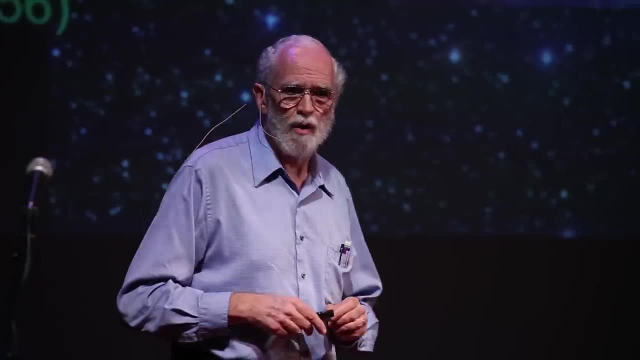 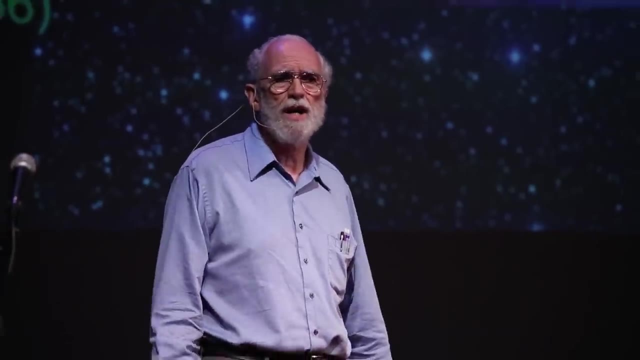 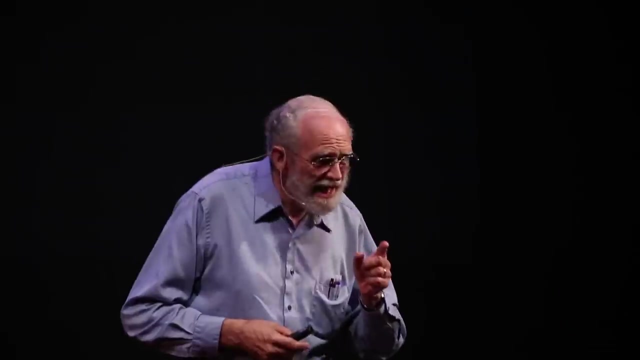 of energy could only be a supermassive black hole, Some kind of hypothetical superstar with nuclear reactions going on inside. it simply could not provide enough energy. Most of you are probably familiar with the concept of energy, particularly if you pay an electric bill. Well, where does the electric company get that energy? 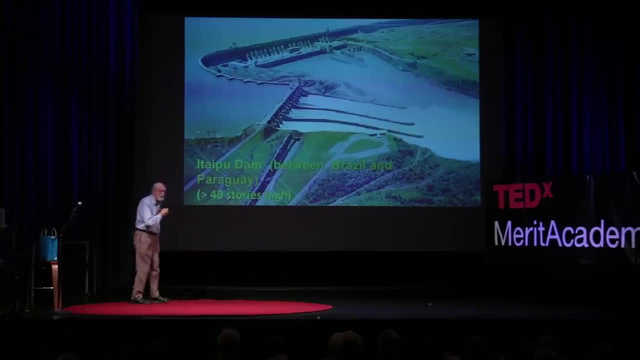 from. Well, one possibility is something like this. This is the Itaipu Hydro Electric Dam. It's very tall. It's about 40 stories from bottom to top there. It's like a big skyscraper At the top of the dam up here. upstream is the water and we say that this water. 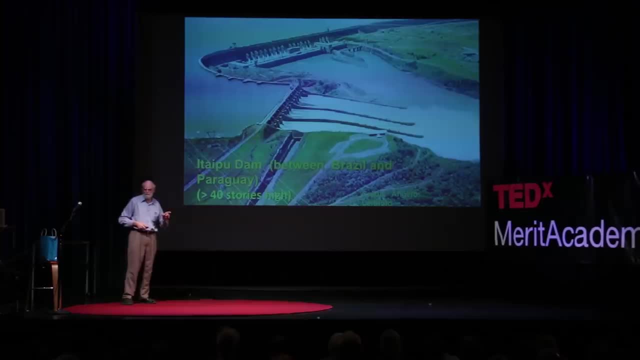 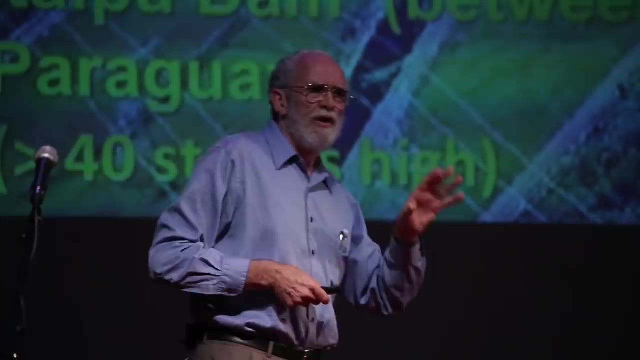 has gravitational potential energy. That means it has the potential to convert and produce other forms of energy. So the water falls over the dam here, falls down 118 meters, and as it does that it is accelerated by the Earth's gravitational speed, and as it gains speed the gravitational potential energy is changed into energy. 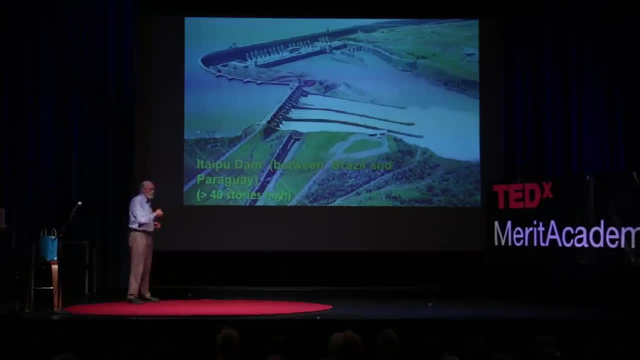 of motion, And that rushing water at the bottom of the dam drives turbines and generators to make electric current, which is then shipped off and heats and lights people's houses and so on. A hydroelectric dam like this is a very good analog of how a supermassive black hole produces energy. 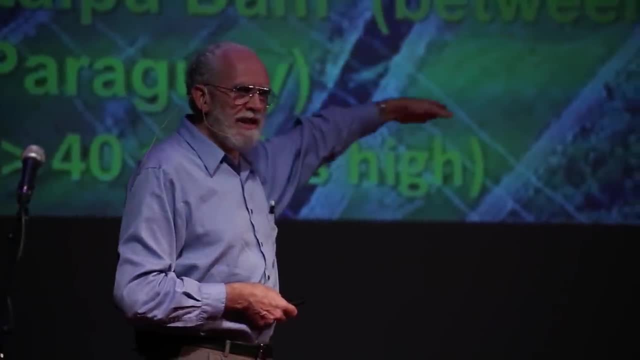 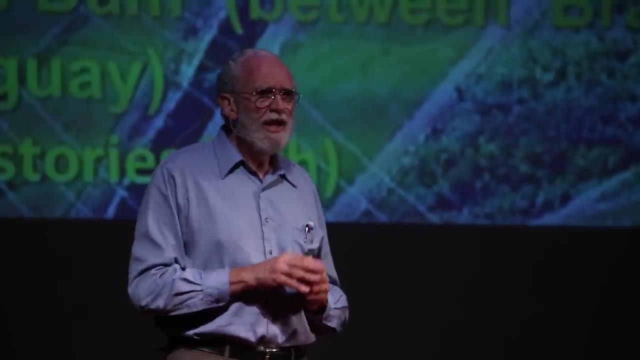 Here the water is only falling down 118 meters. Matter falling into a black hole will fall trillions of kilometers. That's further than the outer regions of the solar system, a good fraction of the way to the nearest star, And it's being. 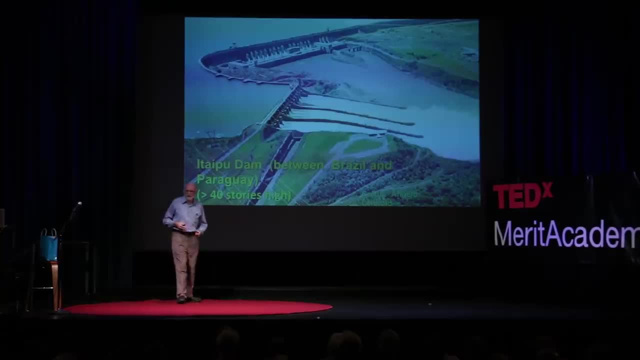 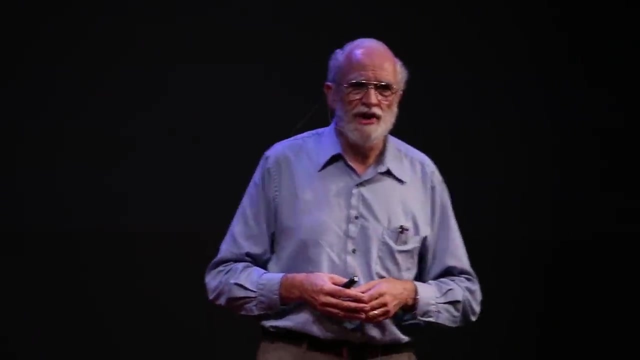 accelerated not by the gentle gravitational pull which is holding us down on our seats right now. It's being accelerated by the tremendous gravitational pull of the black hole. If we calculate how much energy is being produced there for, let's say, one kilogram of material falling into a black hole, it's enormous. It's more than 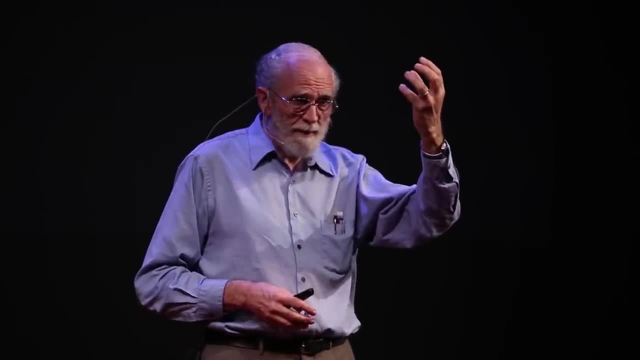 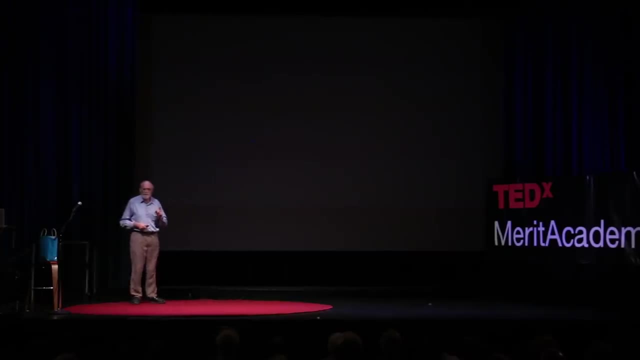 a nuclear explosion of this material would generate. Well, a mere five weeks after Hoyle and Fowler had published their paper, the same journal carried some papers that identified this object. It's called 3C273,. looks like a bright star and indeed that was what people had. 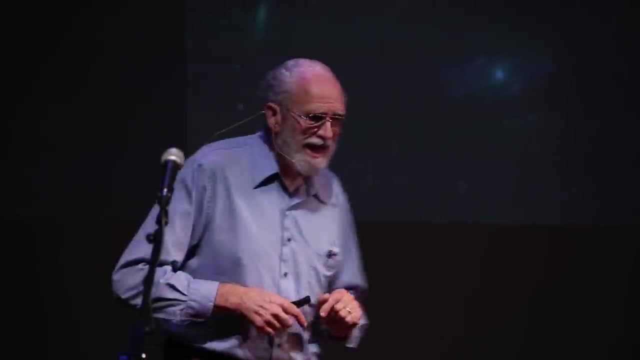 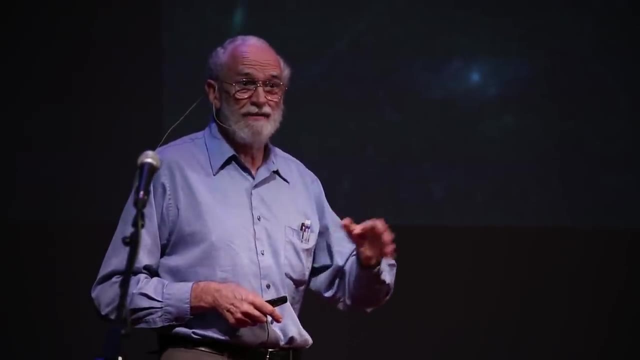 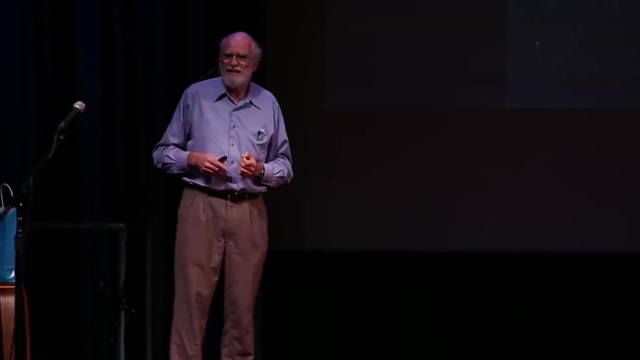 previously thought it was, But astronomers at Caltech showed that this is in fact a distant active galactic nucleus and it's very bright and it's very far away and the brightness of this is more than hundreds of times greater than the brightness of an entire bright galaxy of a trillion stars We can. 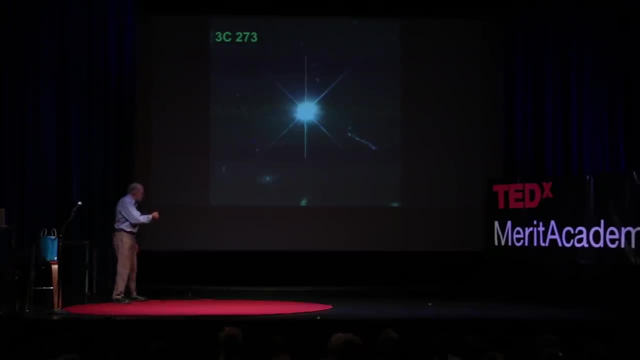 appreciate that in this Hubble Space Telescope, We can appreciate that in this Hubble Space Telescope, picture up here, These little blurry patches which you might not be able to see over here, those are entire galaxies like our own, But just look how bright. 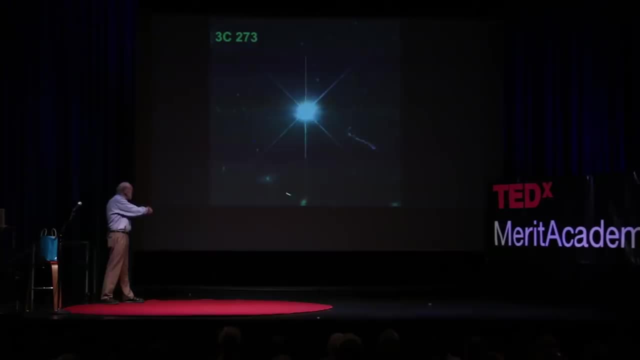 3C273 is. It's brilliantly bright here compared to these ordinary galaxies over here. It's so blindingly bright that we can't even tell that it's located in a galaxy there. That, of course, caused enormous excitement among astronomers and pretty. 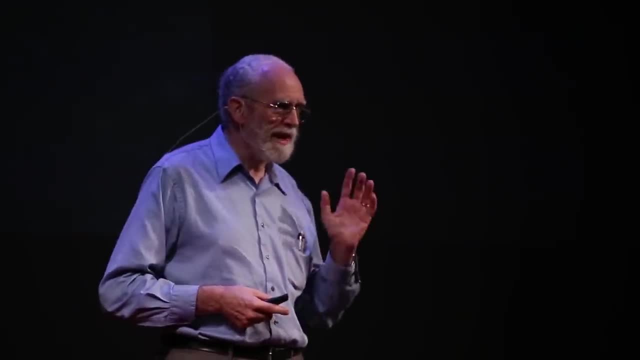 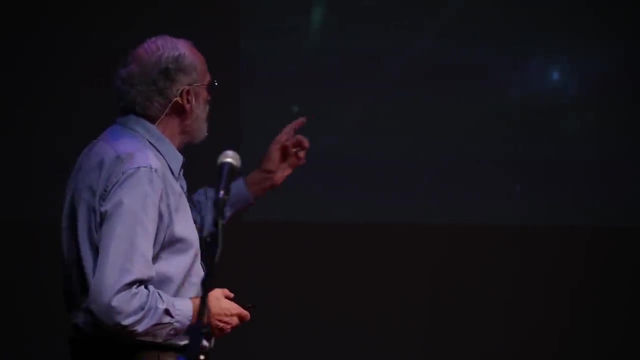 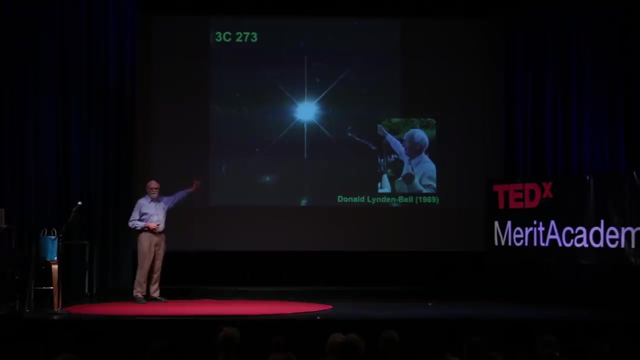 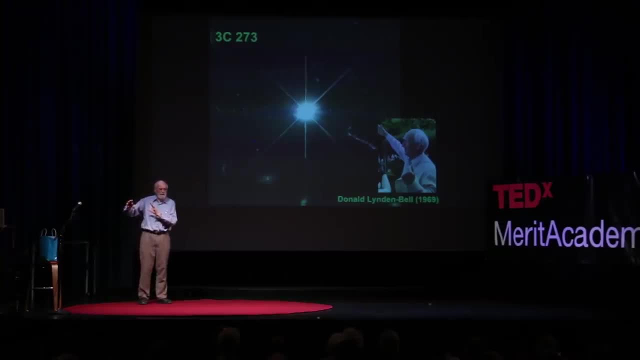 3C273 far away in the distant universe in the past, were being powered by supermassive black holes, then in nearby galaxies there must be dormant black holes- black holes because a supermassive black hole is simply not going to go anywhere overnight and a 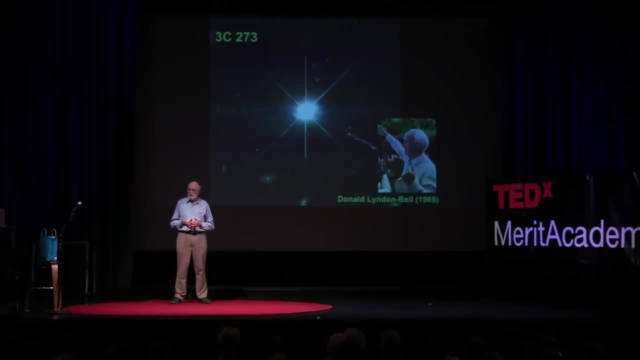 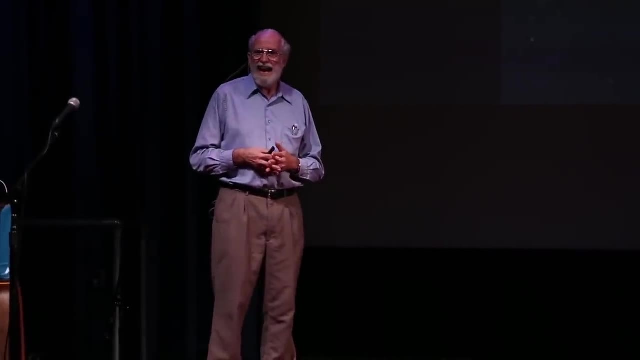 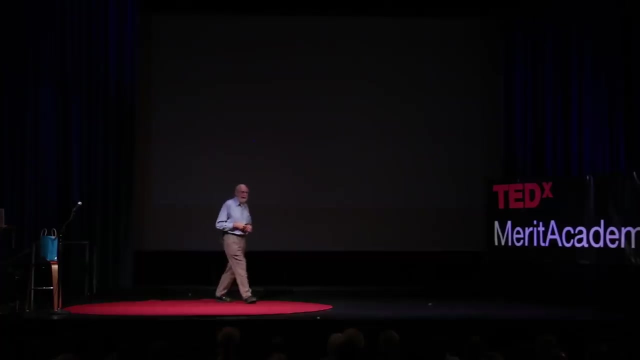 large body of research, continuing down to this present day, by many astronomers, has shown that this is indeed the case. we now think that every massive galaxy has a supermassive black hole in its center. the nearest and best example of this is actually our own galaxy, the milky way, the center. 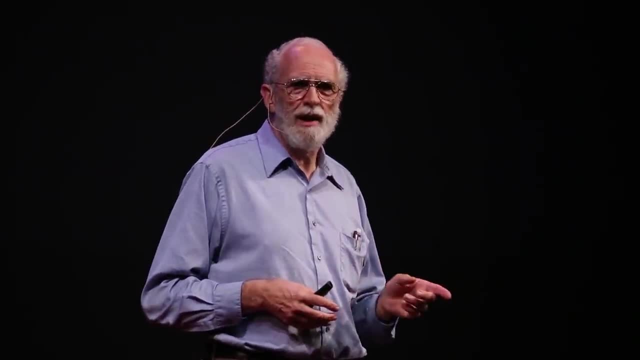 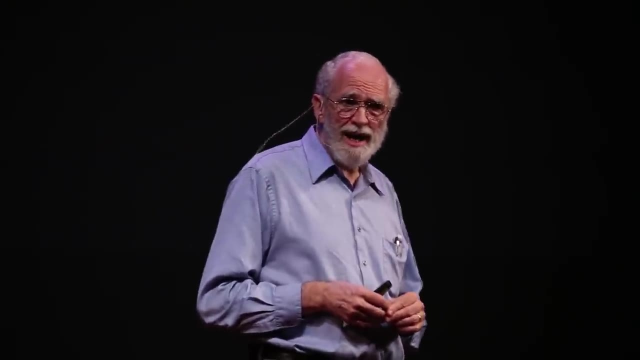 of the milky way. the nucleus the milky way is about 25 000 light years away in the direction of the constellation of sagittarius, but, uh, you will not be able to see it with your eye because there's a lot of dust in space. in the way, however, very large telescopes using infrared 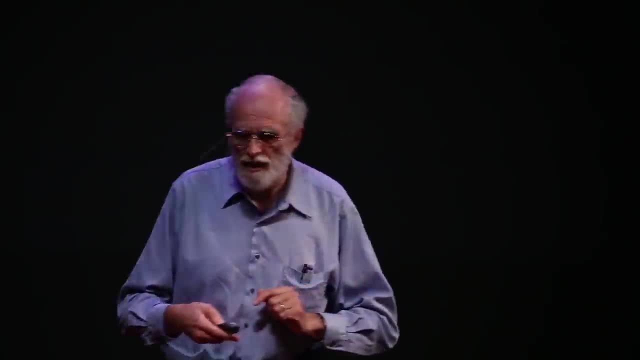 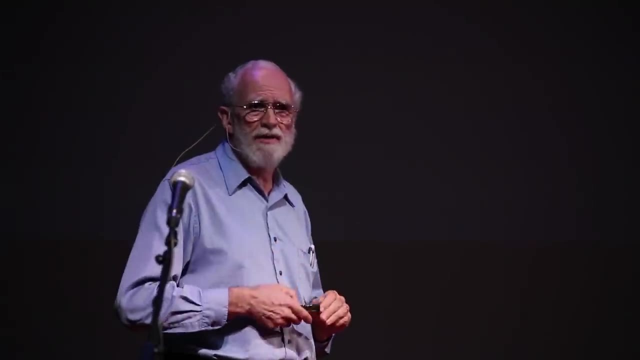 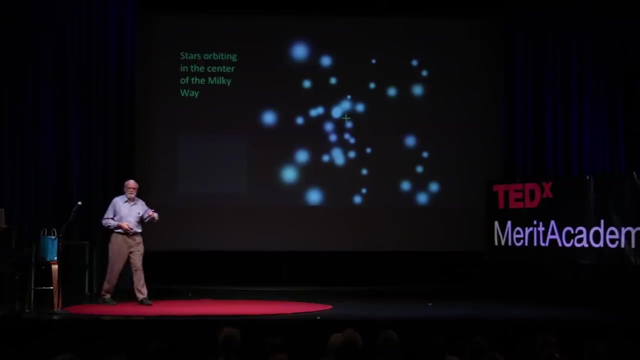 cameras can penetrate the dust and get us pictures of what's going on there. and i want to show you a time-lapse movie which is based on images taken by the european southern observatories, which is based on images taken by the european southern observatories very large telescope, or vlt, in chile. notice, there's nothing at the cross there. 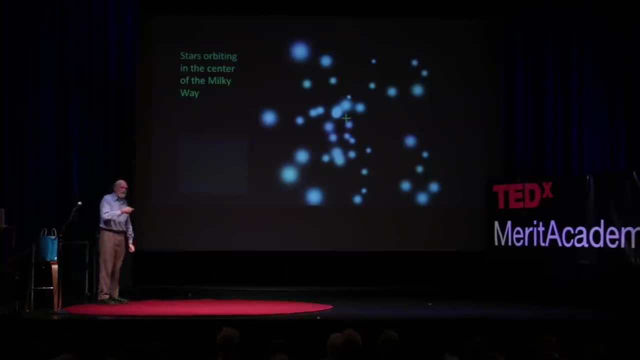 notice that and each one of those blobs there's a star and when i click to start the movie, then the date of observation- if you're wondering when it was- will appear up there. okay, so you can see that the stars are moving around. this is from year to year here. 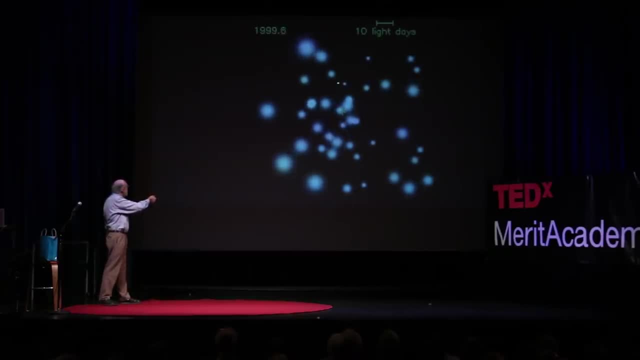 and, and they're moving fastest around this cross in the middle. here let's zoom in on the cross. what these stars? they're going around in elliptical orbits there and let's watch again to this star number two up there. astronomers have really exciting names for stars. here comes star two, comes around here. zips round that cross at high speed there. well, we. 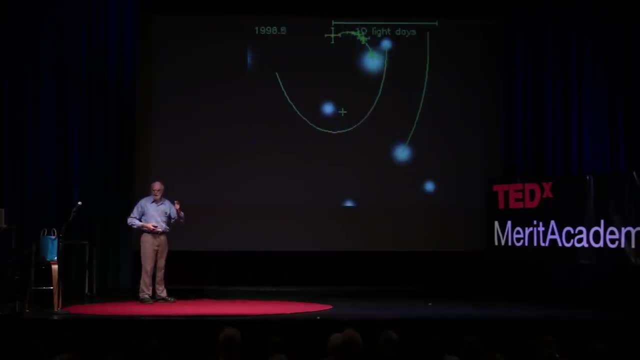 can use Newton's laws of motion, Newton's law of gravity to calculate what force you need to make that star swing round like that And how much mass is needed if it's done by gravity, which it is, And that comes out to be over. 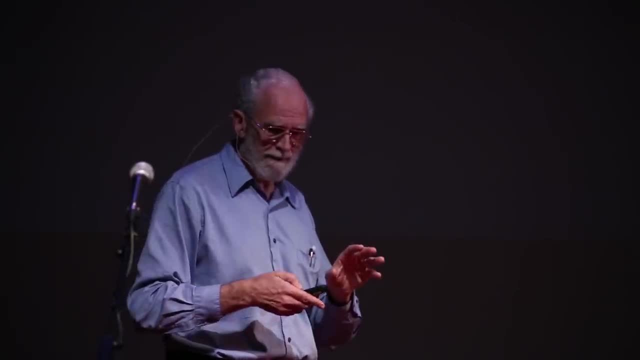 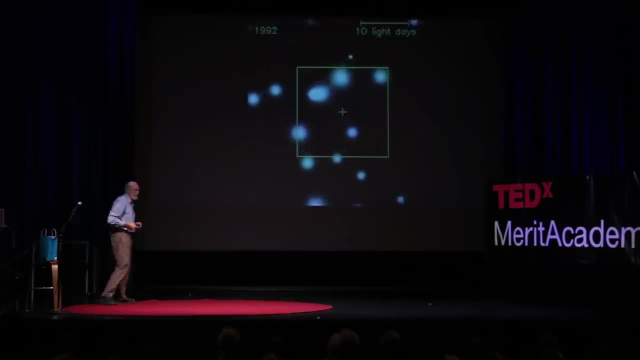 4 million times the mass of the sun. Well, notice the obvious thing there: There isn't anything at the location of the cross there If those 4 million solar masses were in some kind of hyper-superstar powered by nuclear reactions. 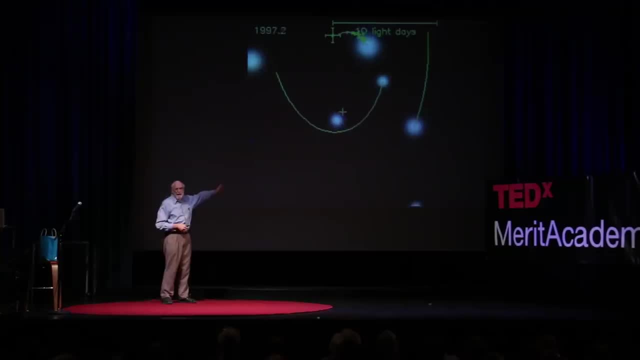 as our sun is. that would be a blindingly bright star, So bright that that picture would be completely washed out and white and you wouldn't be able to see anything up there. Instead, the stars are orbiting around 4 million solar masses of. 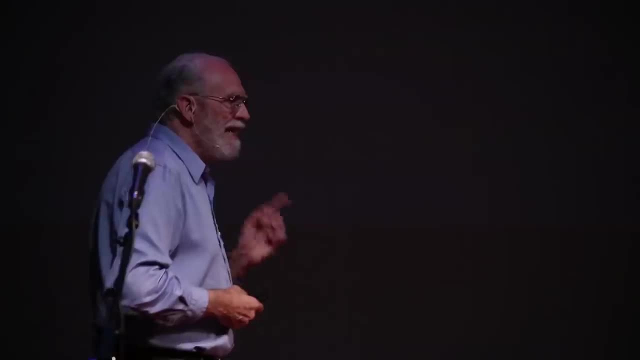 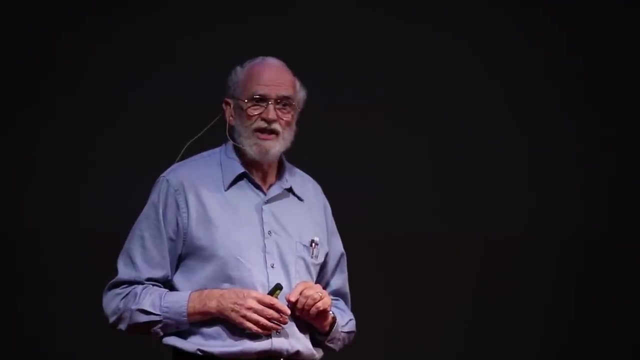 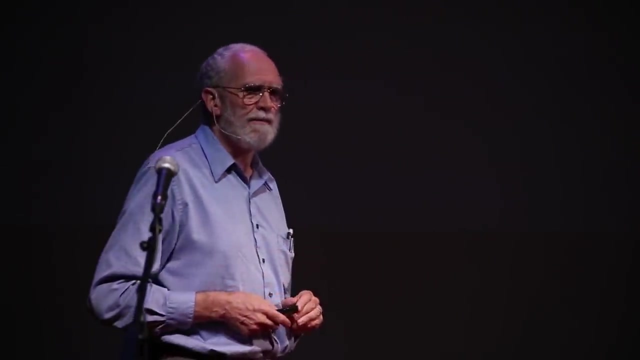 darkness over there. These observations are our clearest proof that supermassive black holes do indeed exist. There's now no reasonable doubt that in the nuclei of galaxies there are supermassive black holes. Well, how do you feed a black hole? 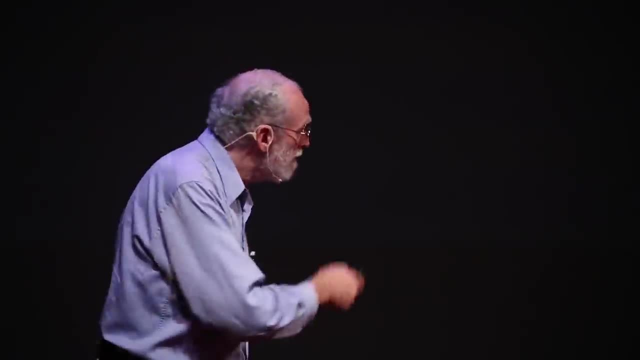 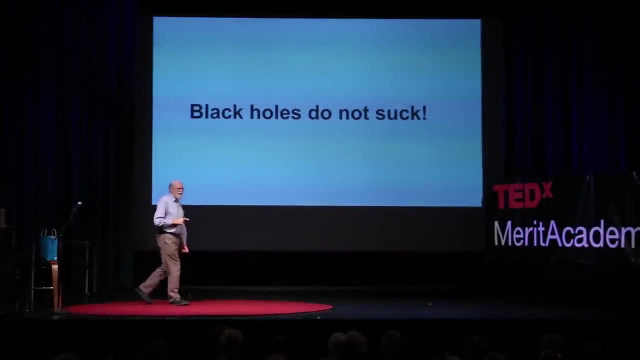 Let me tell you something about black holes. Black holes do not suck. Black holes are not some kind of cosmic vacuum cleaner going around sweeping up, sucking up everything around them. It is, in fact, rather hard to go into a black hole. 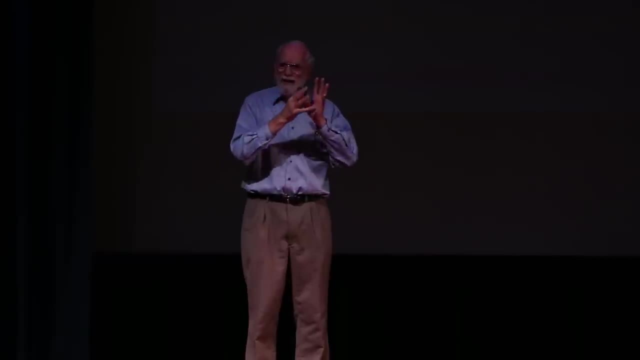 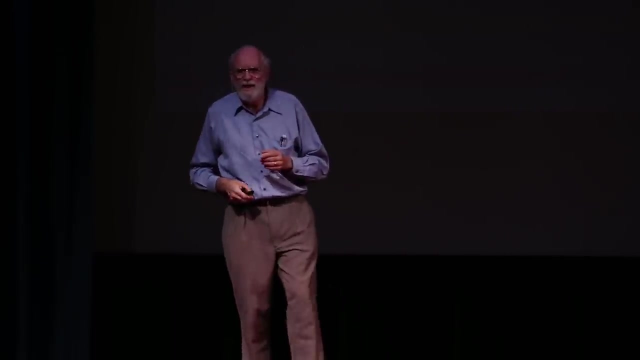 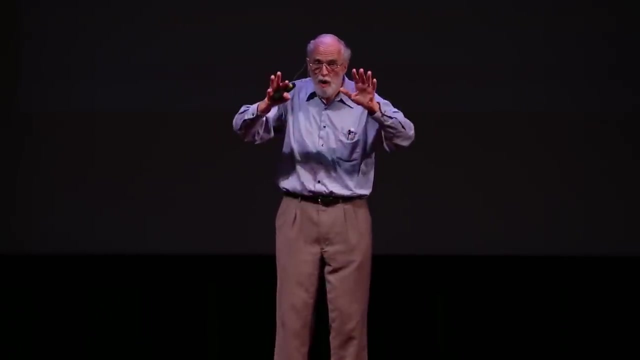 The reason for this is that, except when you're extremely close to the black hole, gravity of a black hole is pretty normal. It's just like any other gravity in the universe. The Earth is orbiting the sun. If the sun were suddenly to turn into a black hole- and don't worry, it won't- 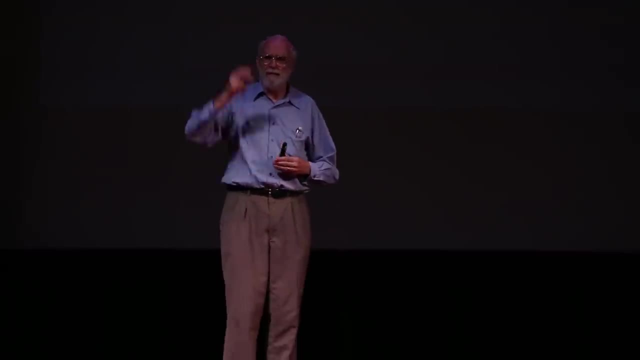 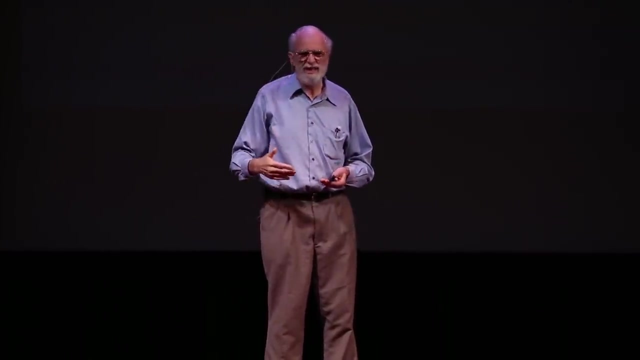 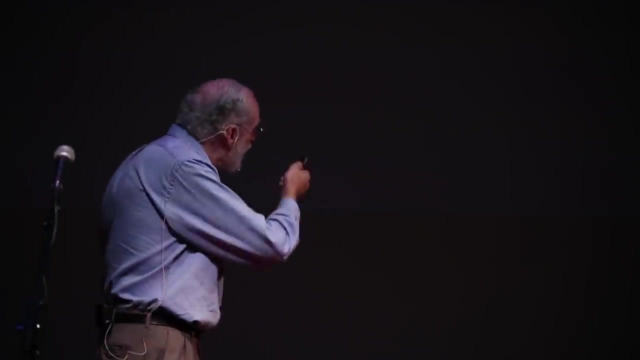 But if it did, if the sun suddenly became a black hole, well, the Earth would just keep on orbiting around the sun. It'll be dark, that's all, but the Earth would keep going around in the same orbit. Let's watch, go back to our little movie of the center of our galaxy and zoom in again. 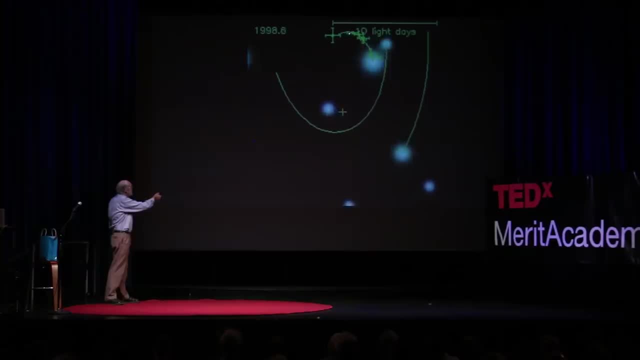 And again, let's watch this star 2 at the top here. Go slowly first, then a bit like Halley's comic coming around the sun, It speeds in and zips around There. the important point here is star 2 there. watch it again is not getting sucked into the black hole. 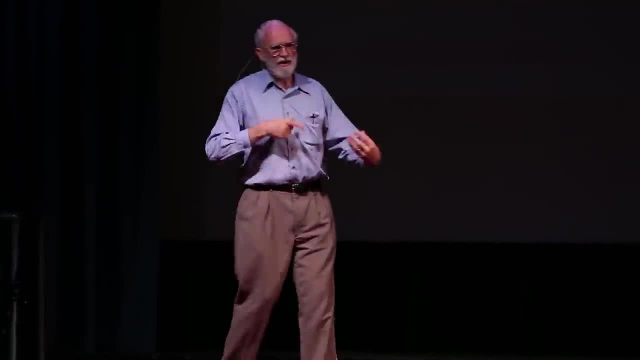 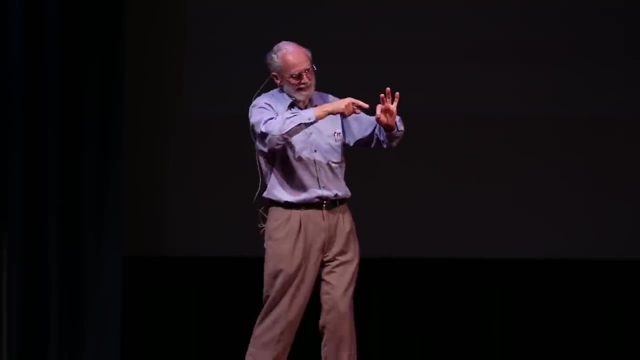 To go into a black hole, that star would have to be on a direct collision course with the black hole, And that's probably not going to happen because the black hole is really small. So it's going to miss and it's going to go flying off. 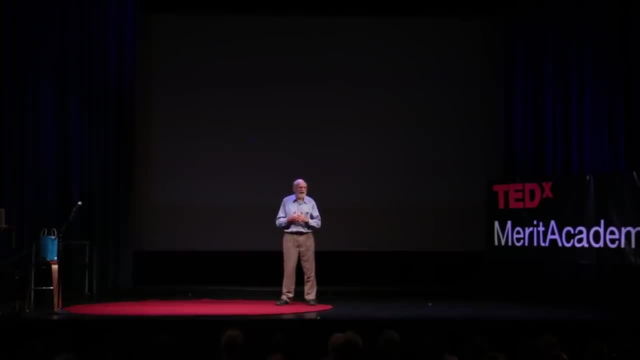 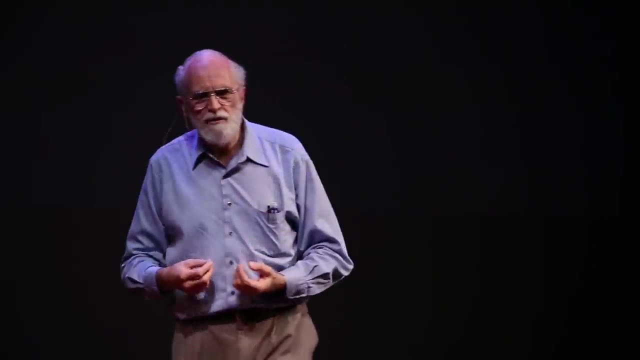 This matter going to black holes is mostly gas, almost entirely gas, And the thing about gas is gas doesn't easily, easily pass through gas. If you've seen a couple of fires burning with columns of smoke. when the smoke comes together, it doesn't pass through like this and keep on going. 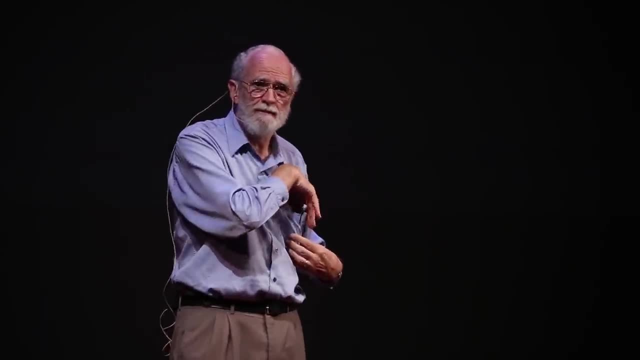 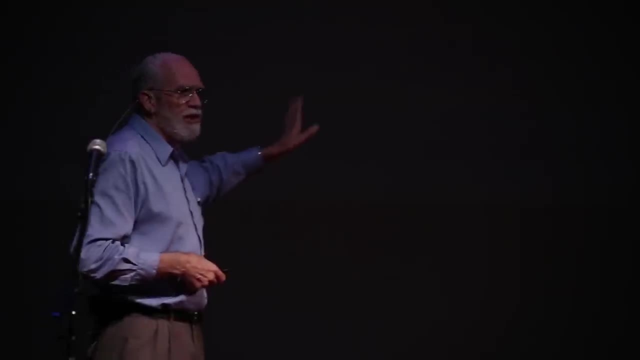 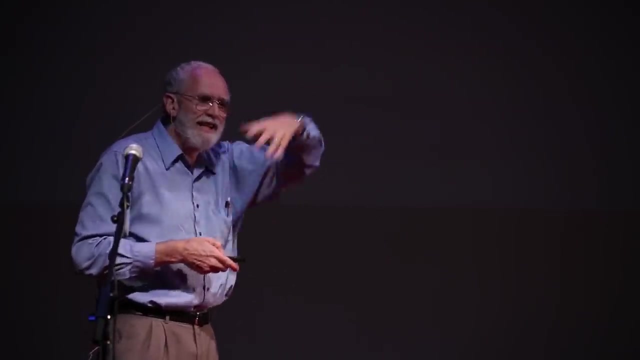 It comes together and it swirls together in one column of smoke. Well, Donald Lyndon Bell recognized that gas that was falling in towards a supermassive black hole was going to end up swirling together and end up spiraling around it and settling. 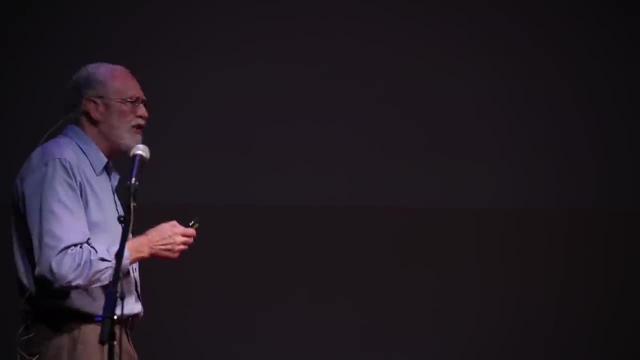 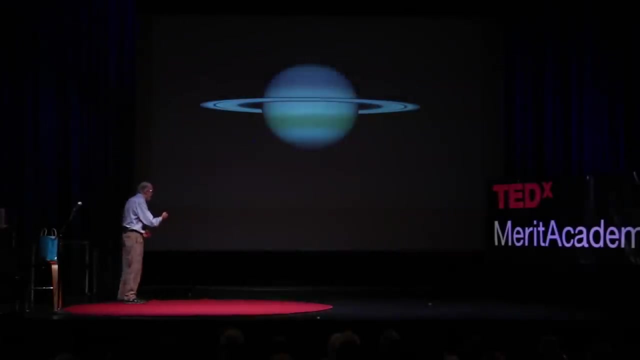 down into what we call an accretion disk. Now, disks are quite common in astronomy. This is the best-known nearby example: the rings of Saturn. The rings of Saturn are particles of dust and ice orbiting together around Saturn, here in a very thin plane. 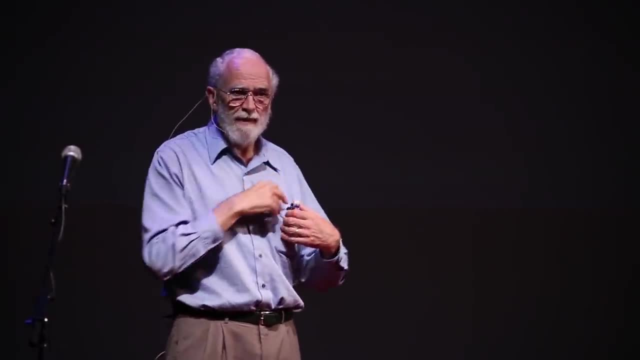 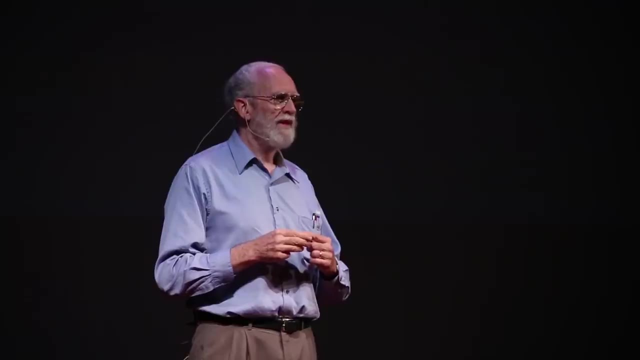 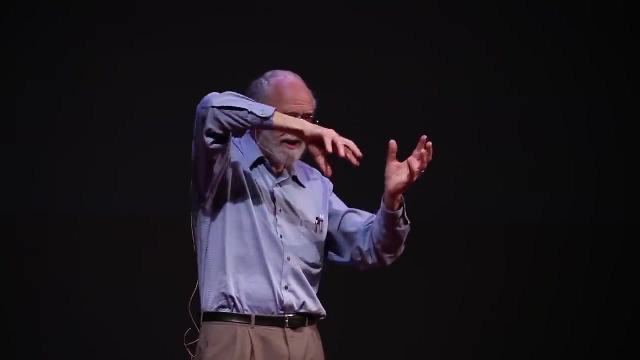 The material going to a black hole is actually not dust and ice, like Saturn's rings there, It's gas. Gases and liquids have a special property that we call viscosity. means that one part of a gas is pulling another part, or one part of liquid is pulling on another. 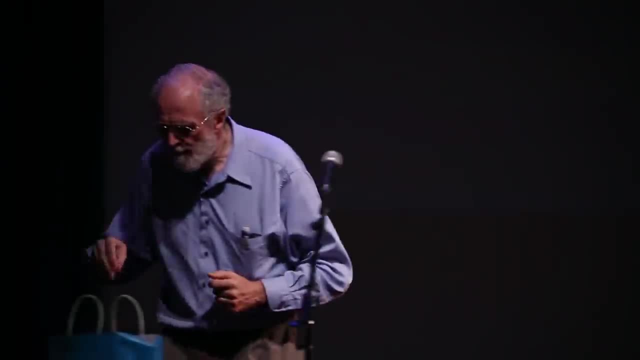 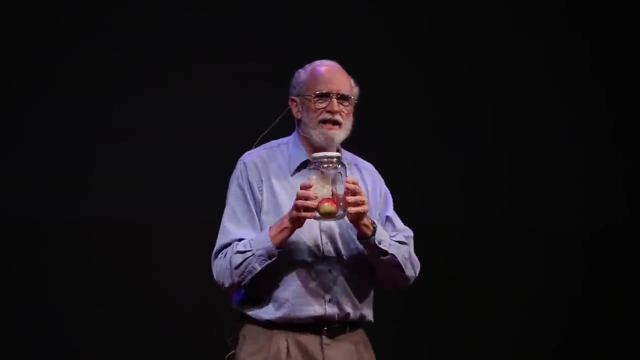 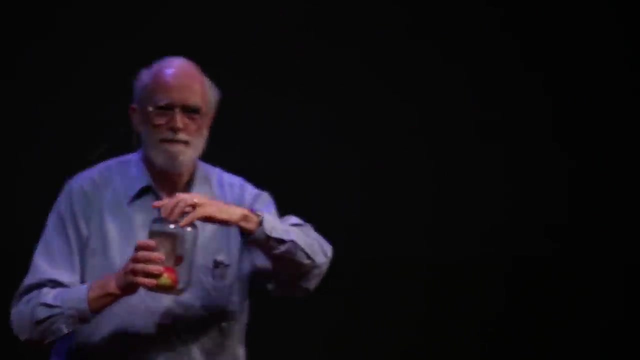 part and I've got a little demonstration to show this over here. So here I have a jar and inside this jar is an apple. I just thought if we're going to do an experiment with gravity, then apple was the right fruit to use. If I take this apple here in the jar, I turn the jar upside down you. 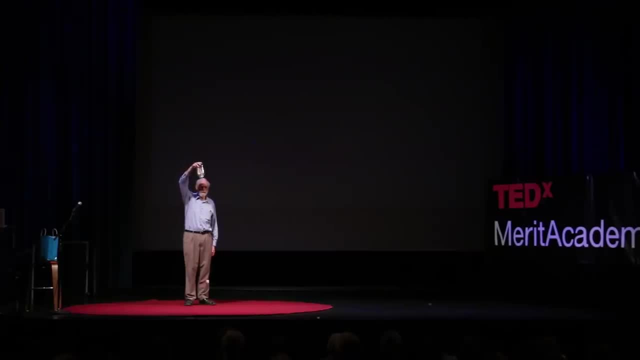 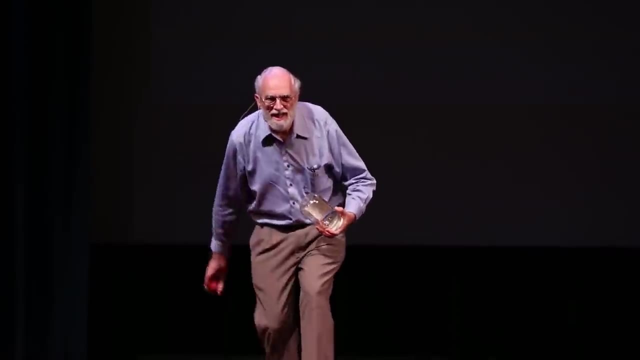 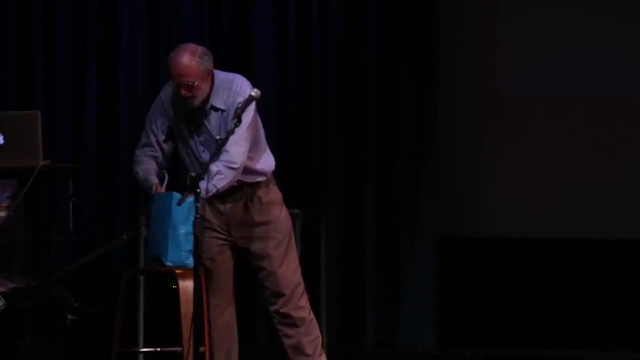 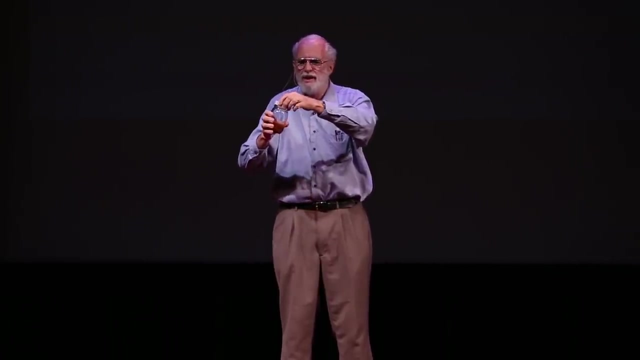 all know what's going to happen: It's going to fall down on the ground. So here we have a fine apple. Who would like an apple? In my other jar over here, I have something different. This is a jar of honey. Organizers wouldn't mind if I tip this honey upside down and put it on the carpet, right? 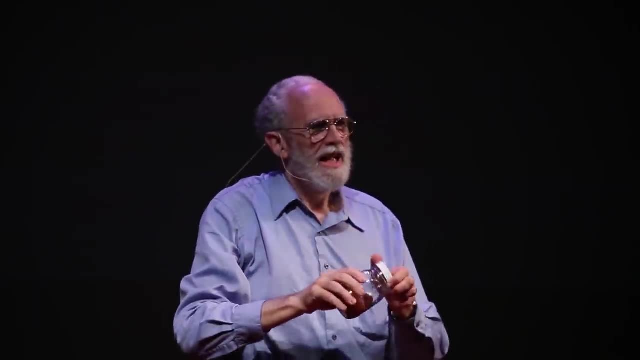 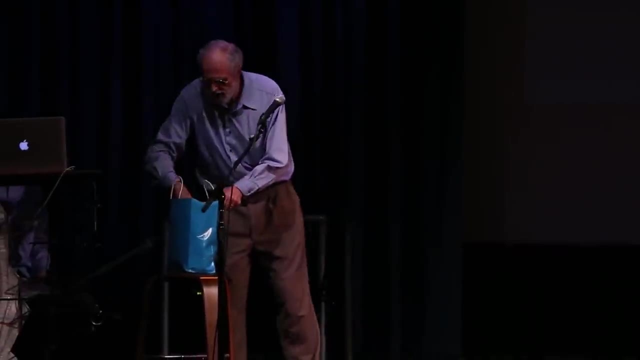 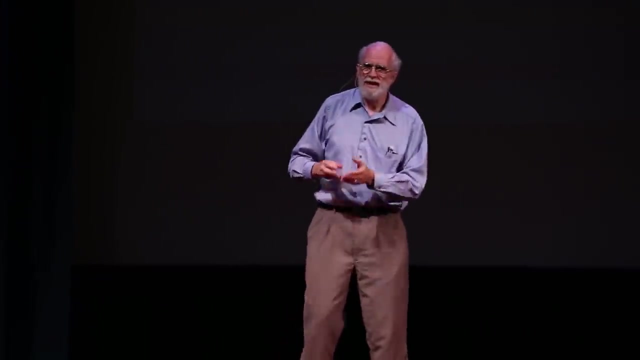 Oh, it's not going out very quickly, is it? That's because honey is viscous and the viscosity of the honey means that there's a blob in the middle which would like to fall down on the floor and make a mess on this nice red carpet here, but it's being held back by the viscosity of the honey, which is. 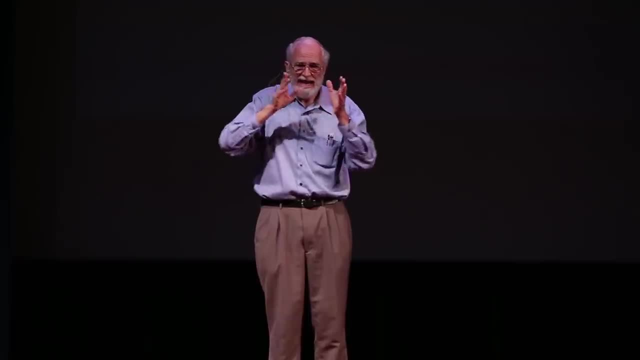 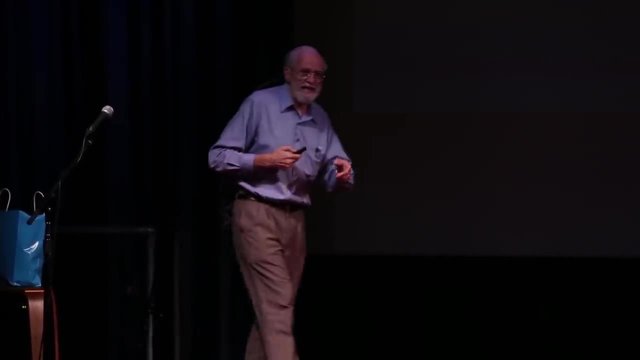 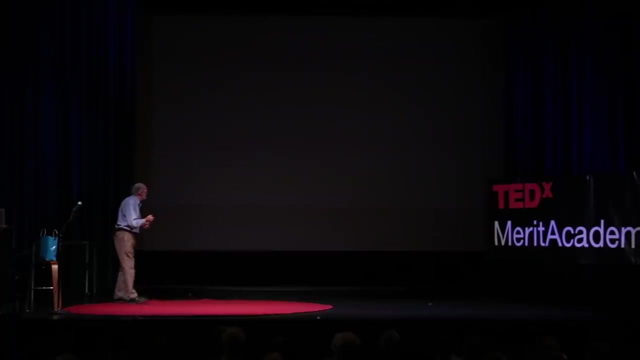 around it, and that honey, in turn, is being held back by the edge of the jar there. Well, a similar thing can happen. The viscosity in the gas is not quite like the viscosity in the honey. It's actually provided by tangled up magnetic fields. But let's have a look at Saturn's rings again. 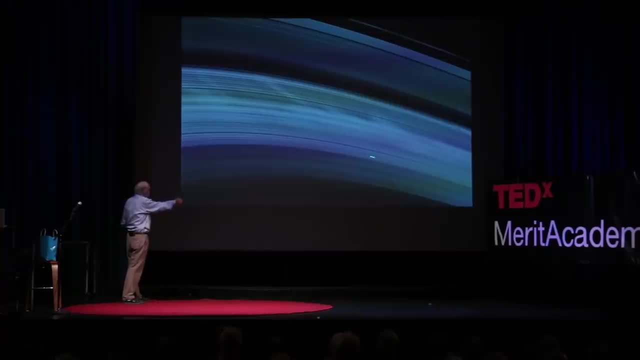 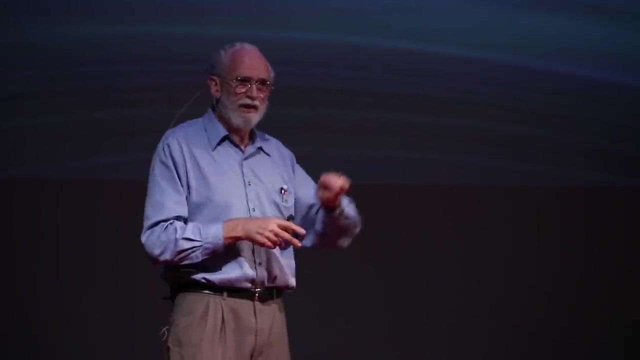 What you can probably tell from this picture here is that the inner part of the rings is going faster than the outside part. You can see it's sort of dragged off here. This is like the planets going around the sun. Mercury, the closest planet to the sun, goes faster than Venus, the next planet out. 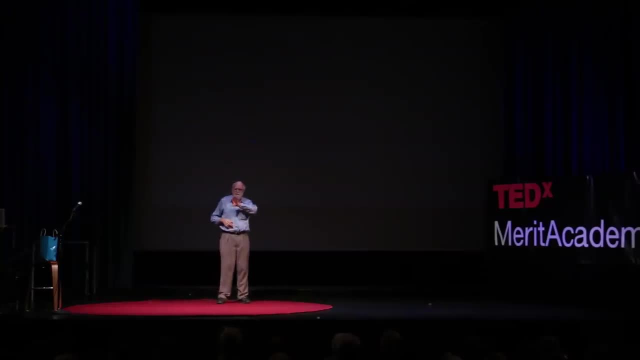 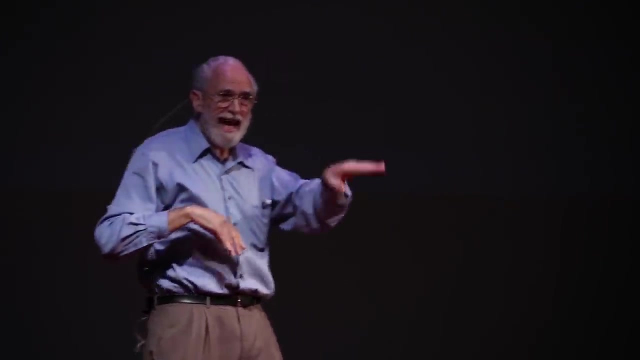 Venus goes faster than the earth, and so on. The gas on the faster orbits is being held back by the gas further out, and that's going to slow it down. It's going to make it go into lower orbit and thus spiral into the black hole. So, Donald, 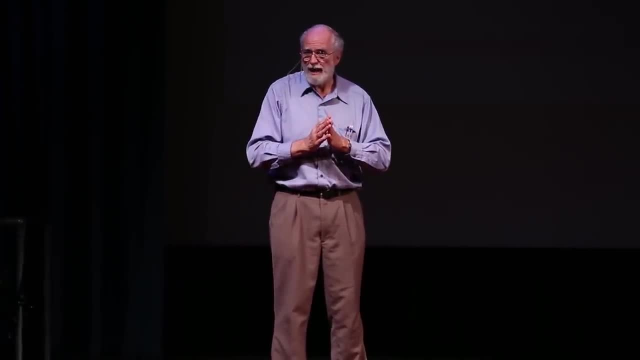 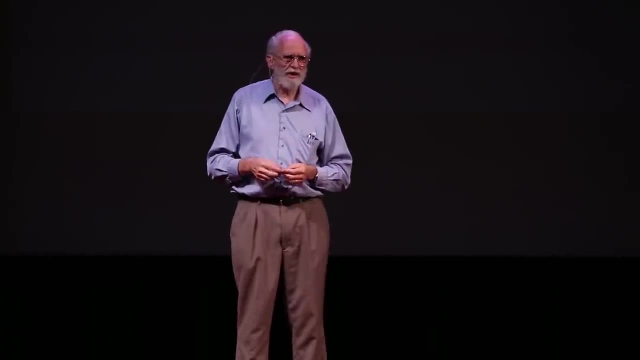 Lyndon Bell proposed that that is how you go inside a black hole. Well, viscosity doesn't just make stuff go into a black hole, It does something else as well, And let's do a little demonstration of the other thing that it does.